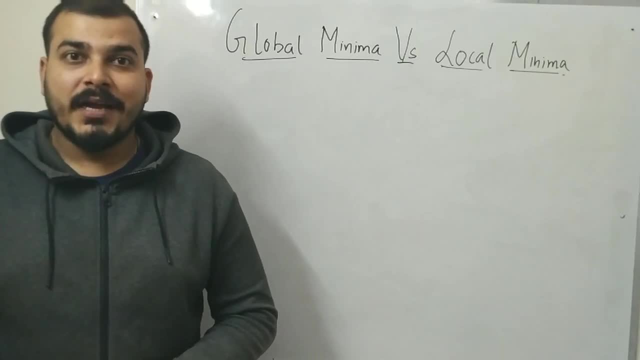 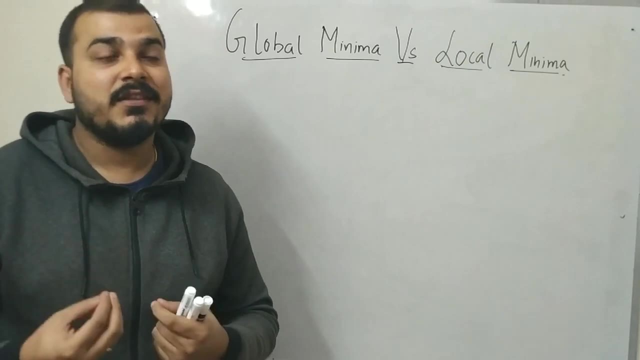 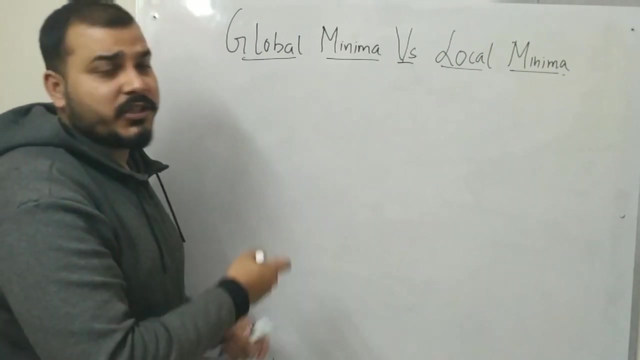 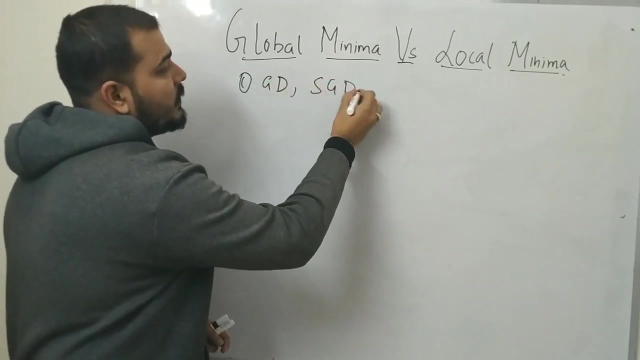 Hello all my name is Krishnag and welcome to my YouTube channel. Today we will be discussing about Global Minima and Local Minima. We will also try to understand what is the basic difference between Global Minima and Local Minima. Let me just rewind some of the topics that we have discussed in our previous class or previous session. First topic that we had already discussed is about Gradient Descent. We have discussed about something called as Stochastic Gradient Descent. 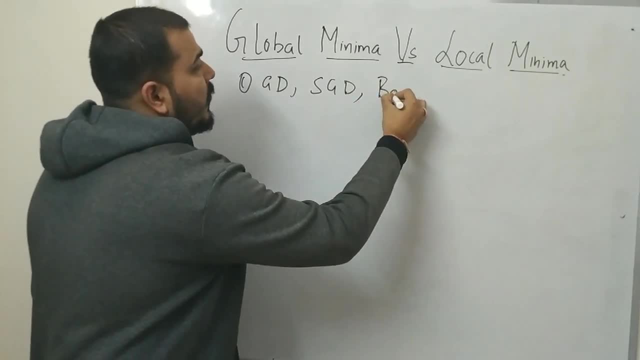 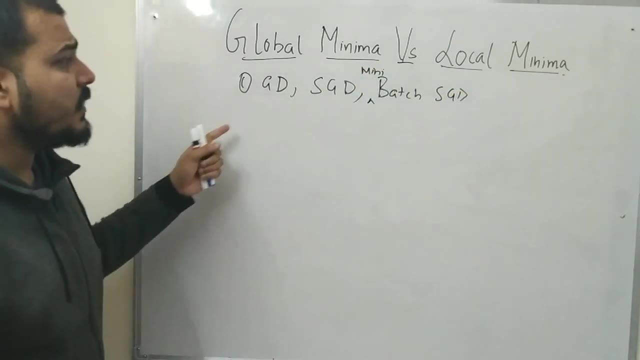 And after this, we had also discussed something about Mini Batch, Stochastic Gradient Descent, So I will just write it as Mini Batch. Now, when we were discussing all these things, we understood why we have to use Mini Batch: Stochastic Gradient Descent. 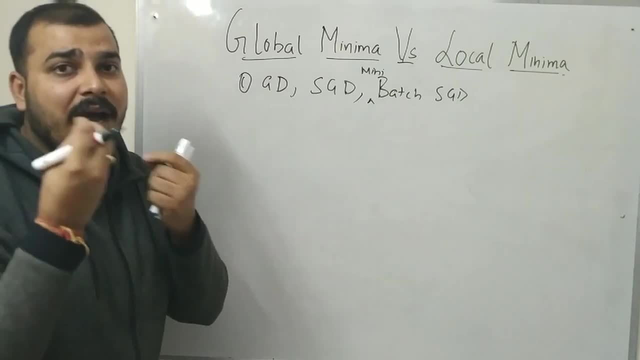 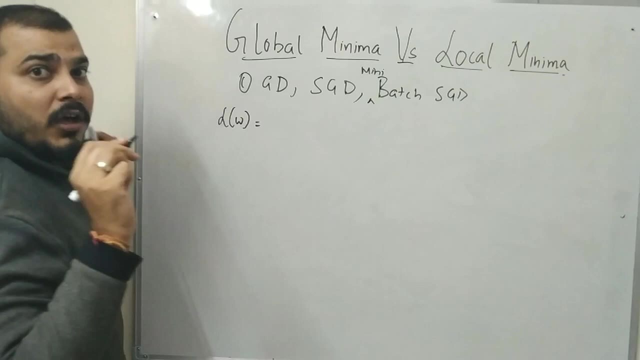 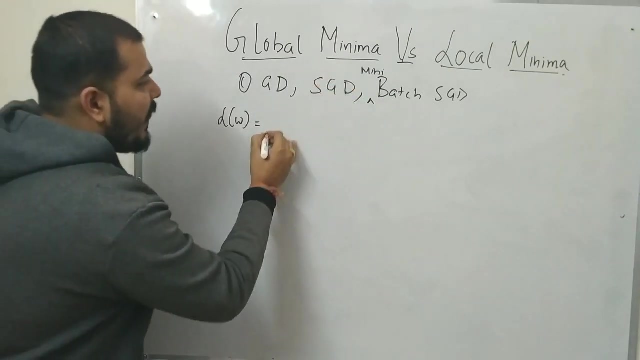 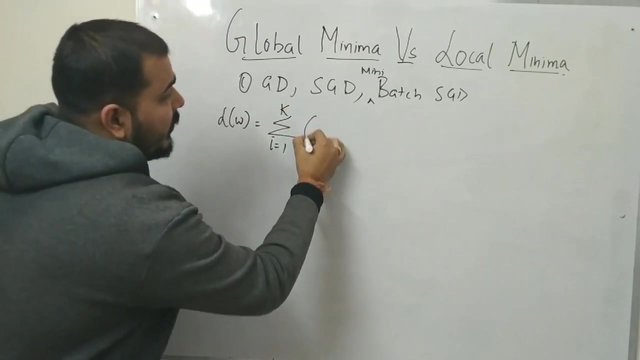 Now understand that during the batch propagation we always have some kind of loss function. So let me just write one of the loss function, So Lfw. one loss function that I have specifically discussed in each and every session is basically called Lfw And for that, if I am using a Mini Batch Stochastic Gradient Descent, the formula becomes: I is equal to 1 to K And I can just write it as: Y minus Y hat whole square. So this is basically my Mini Batch Stochastic Gradient Descent. 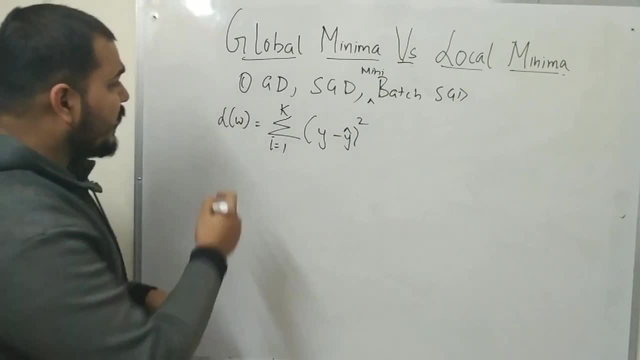 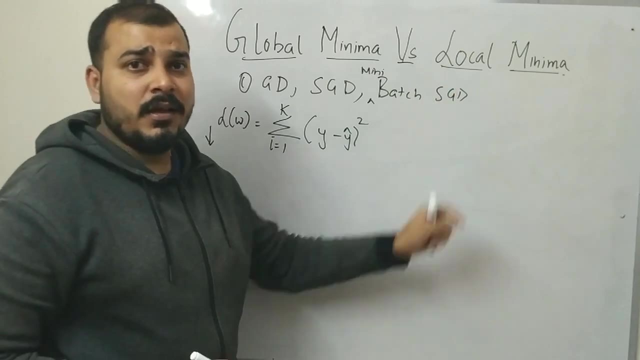 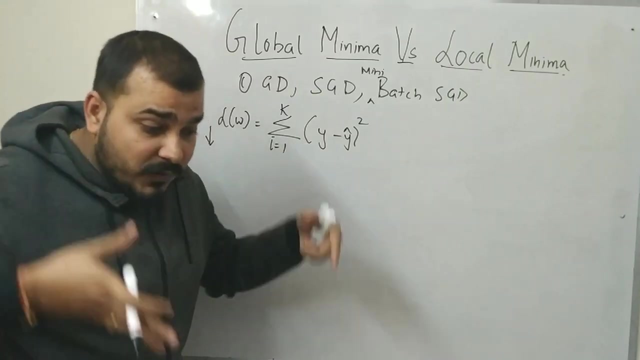 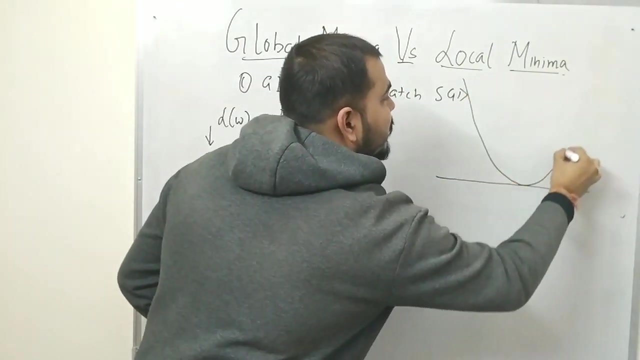 Now let me just go ahead and draw. Now I have to reduce this loss function, And for this I am using the optimizer, which is called as Mini Batch Stochastic Gradient Descent. Always remember this kind of loss. So this loss function will create a gradient descent. I mean the convergence graph as shown as I am trying to draw over here. Now see this: My curve will look something like this: 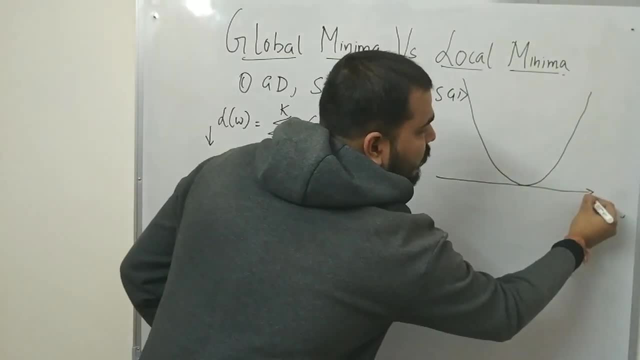 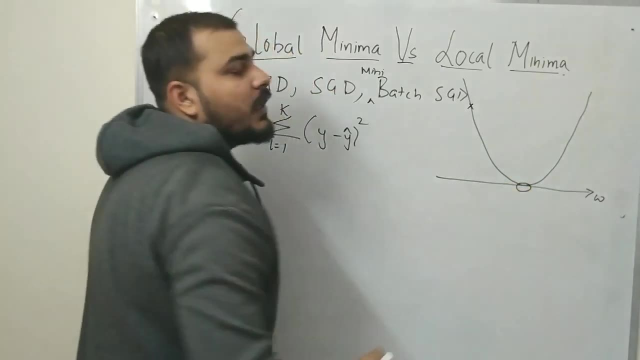 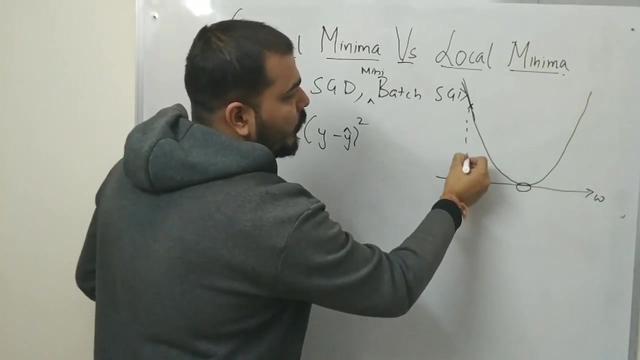 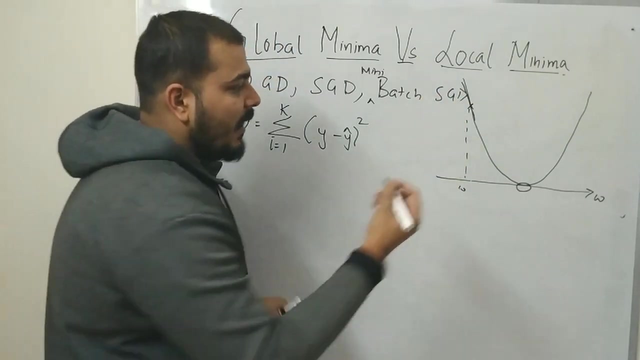 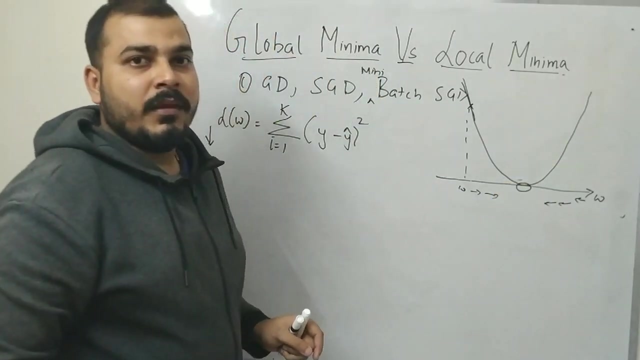 Now this particular curve in the X axis is basically my weights And we know that our weights we have to converge at some specific point at this particular location. Suppose my initial weights is over here. I find the derivative by creating a tangent line. So I get my weight over here. Now, based on this particular point, and if this derivative is positive or negative, I have to basically increase or decrease the weight to come to this particular location. 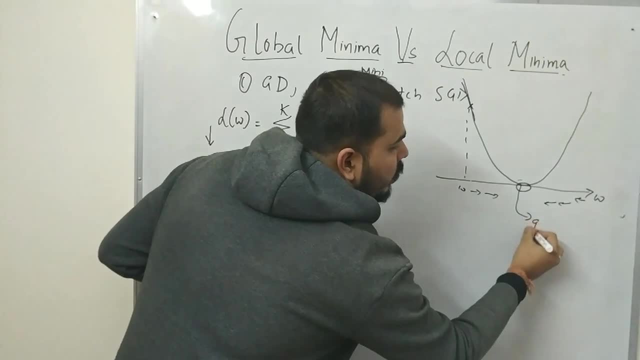 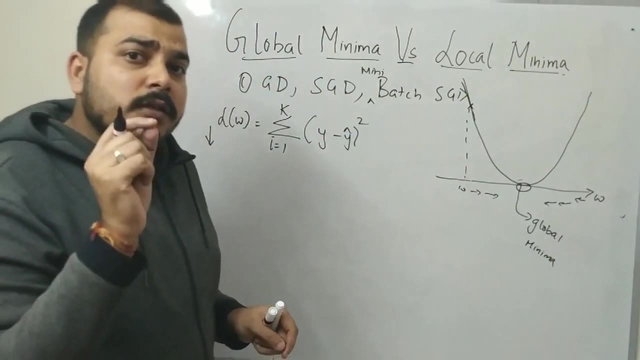 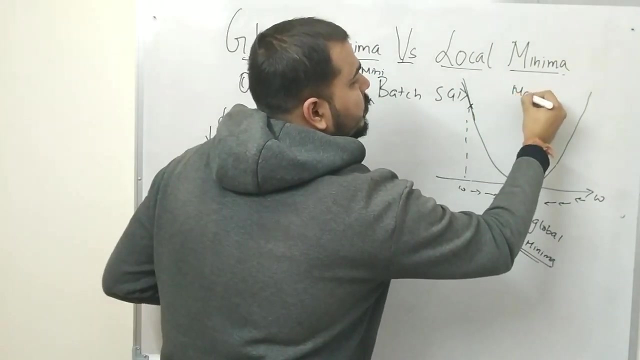 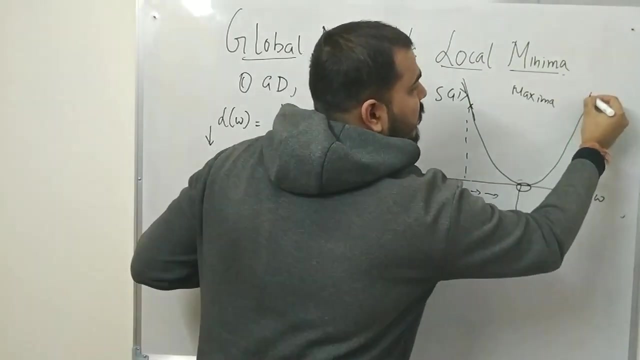 And this particular point is basically called as my Global Minima. Now I would like to introduce you to one more topic. We have discussed about Minima. There is also something called as Maxima. Maxima, in this particular curve, is not present, Because you can see that this line may get extended to any level. 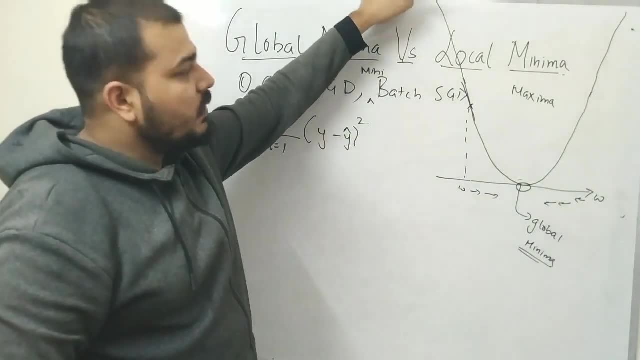 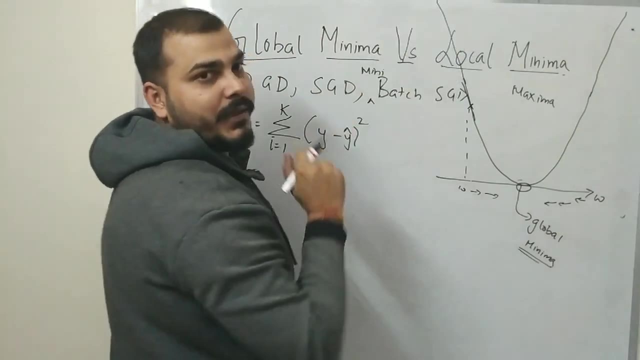 So there is no such stoppage of this particular line. So in this particular gradient descent curve, you will be seeing that there is no such Maxima and it can go up to any height, Whereas in the case of Global Minima It will at least converge at one particular point. 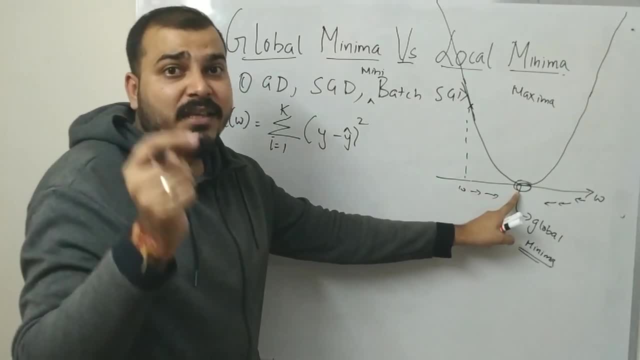 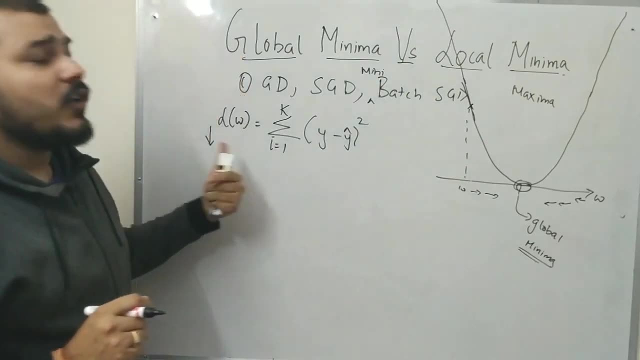 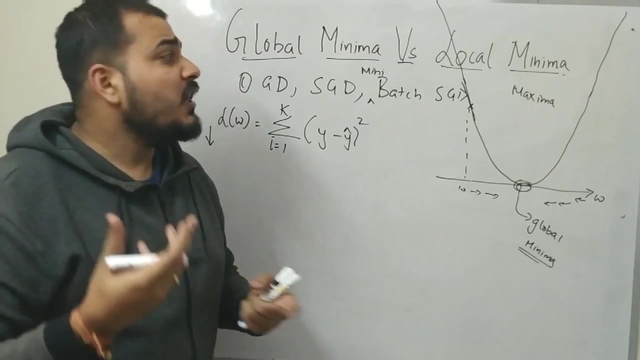 And this particular point will be my best weight- to actually find out the predicted output. Now, this is in the case of this kind of loss function, But in deep learning there are also different kind of loss function which does not create the shape of gradient descent. 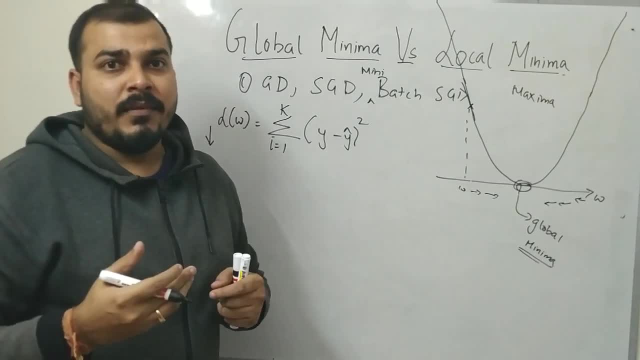 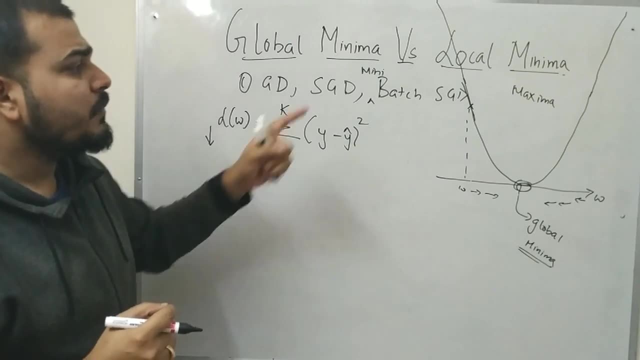 It will be having a different shape And there is where this particular term which is called as loss function, The term which is called as Local Minima, will come into existence. Let me just draw a simple curve once more for a deep learning, for different loss function. 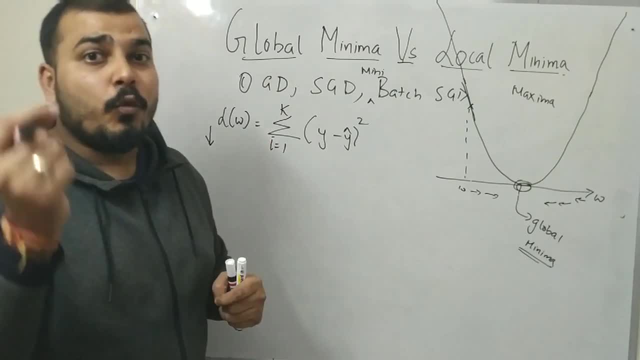 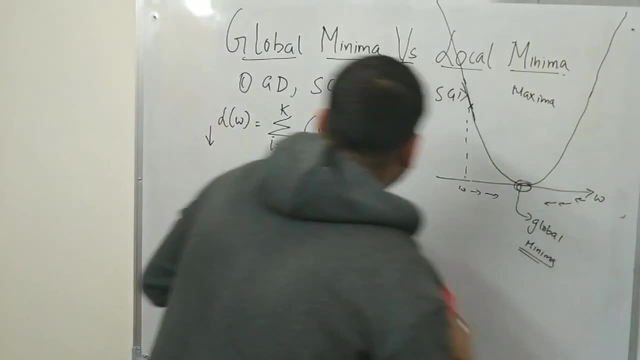 Not for this exactly: loss function, for a different loss function, And what will be those different loss function? I will be discussing that in my upcoming videos. So I am going to just rub this and let me just draw one more curve. Let me just draw one more curve. 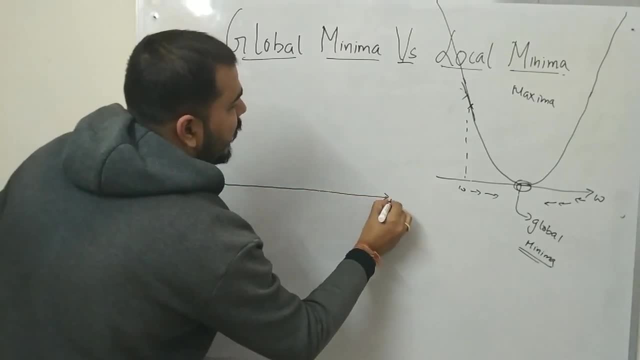 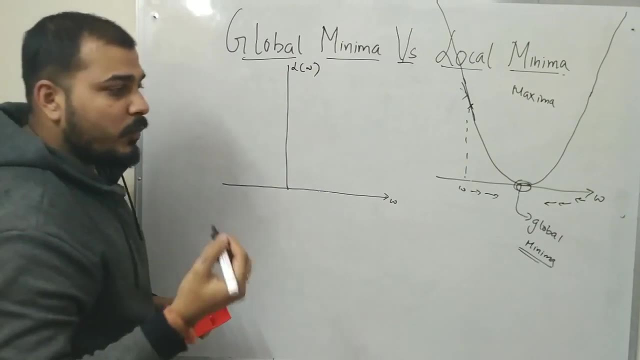 Suppose I draw my other curve again over here In my X axis it will be W And this is basically my loss: L of W, And here you will be observing that there will be some kind of curve which will be created somewhere like this: 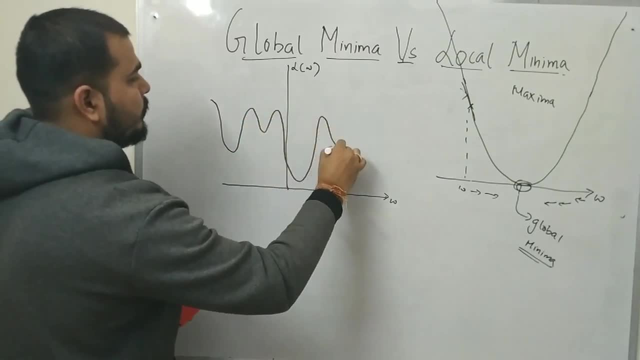 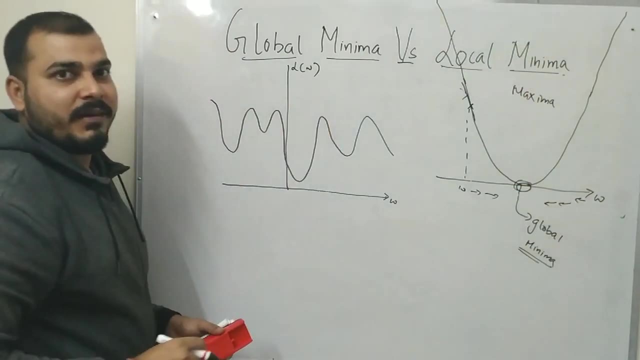 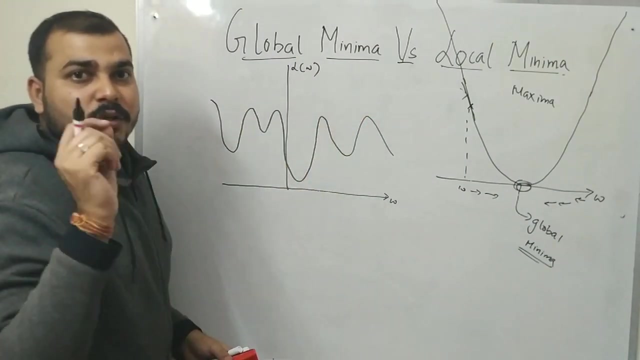 Now, this kind of curve does not resemble this kind of curve Over here. now just try to find out which will be the Global Minima. from this particular diagram, You can observe that which will be having the lowest curve, which is converging completely to the down. 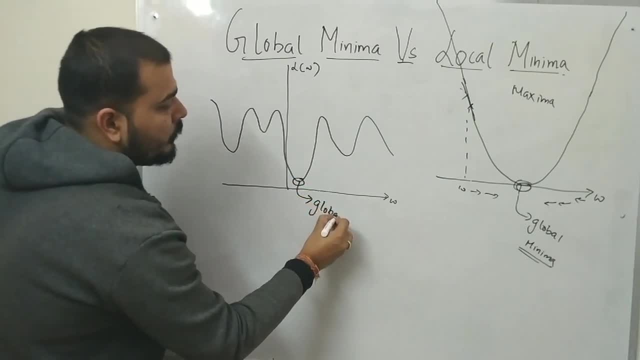 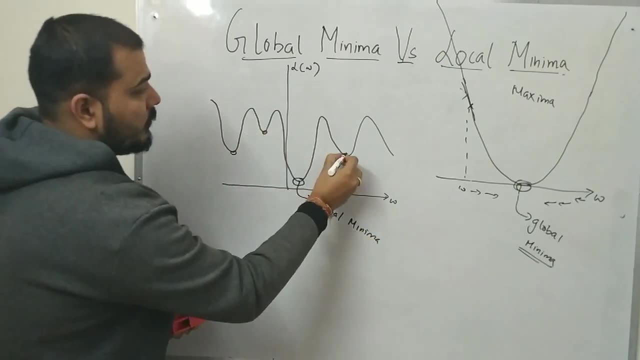 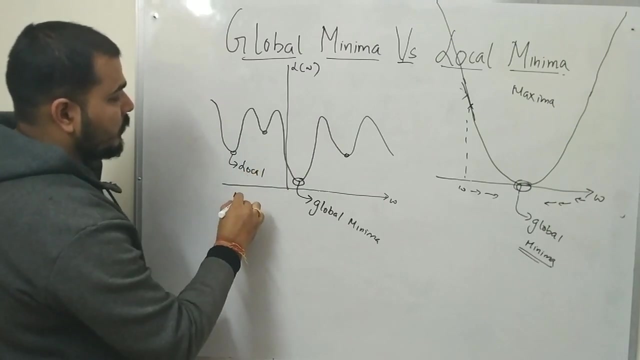 This point will be actually called as your Global Minima, Whereas now next question arises: what will be this point called? as There are so many points over here, These all points will be basically called as Local Minima. Why it is called as Local Minima? that you need to understand. 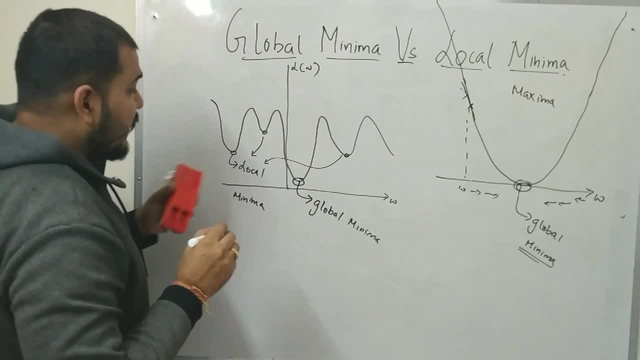 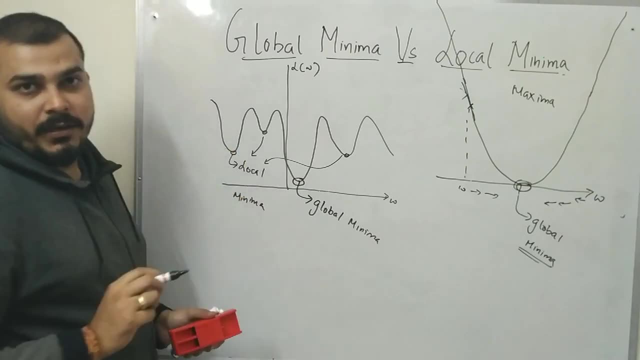 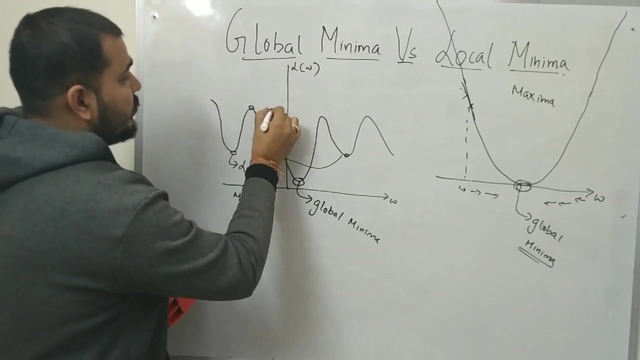 It will be similarly called as Local Minima. It is basically called as Local Minima because in this particular locality, this is the best convergence, This is the best Minima point. That is why it is basically called as Local Minima. Now the next question arises: what will be this point called as? 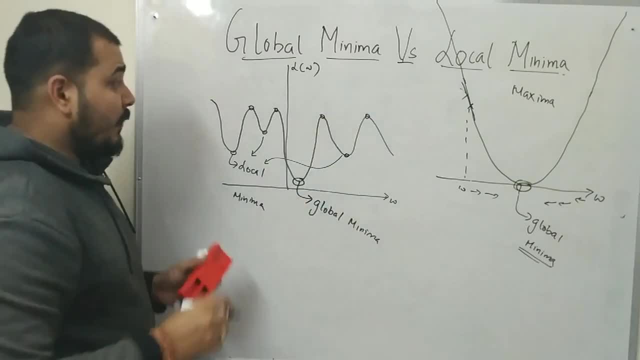 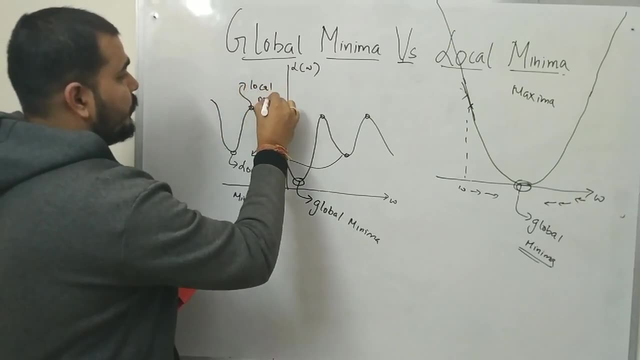 Because here also I am having some points, And why I am specifically taking these points. I will just tell you in a while. These points will basically be called as my Local Maxima. Local Maxima Now. what will be Global Maxima then? 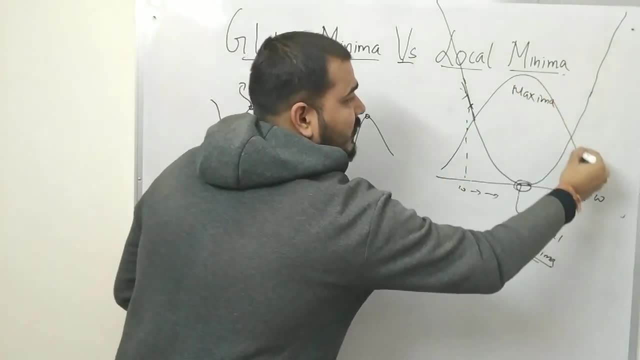 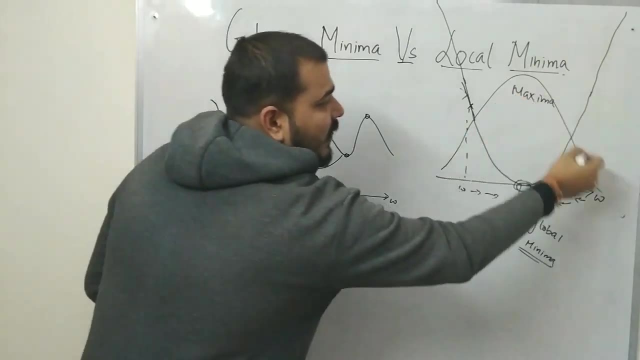 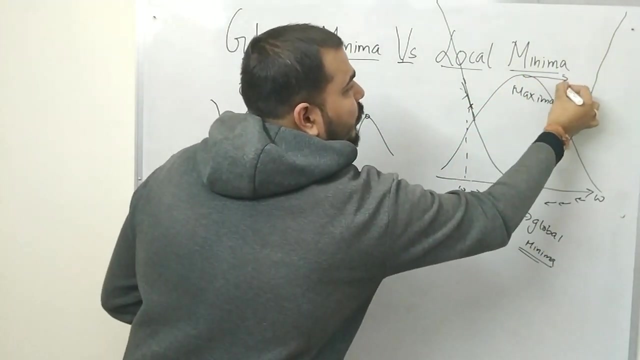 Just consider that I am trying to create one more curve which looks like this At this particular specific diagram. here you can observe that I don't have any Global Minima for this curve, Because it is not converging anywhere. So here this position will basically be called as my Global Maxima. 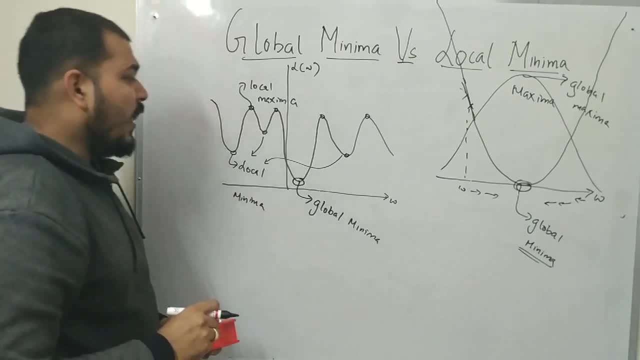 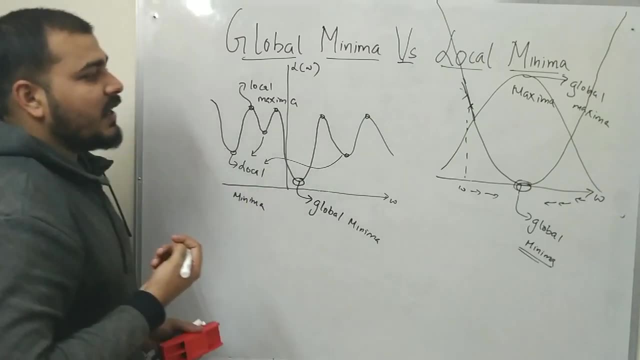 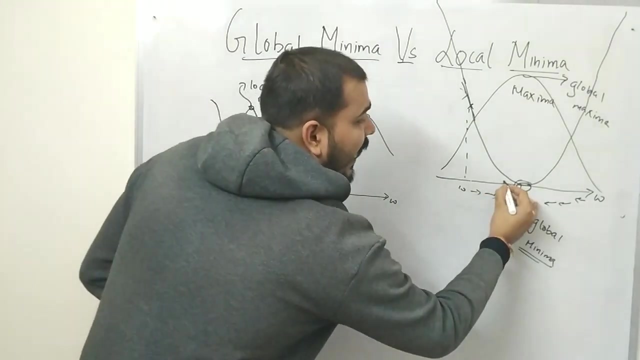 Global Maxima. Now, why are all these points very, very important? Okay, So let us just understand. Always remember, guys, whenever there is a Global Minima, or whenever there is a Local Minima, Whenever I go and try to calculate the derivative at this point, 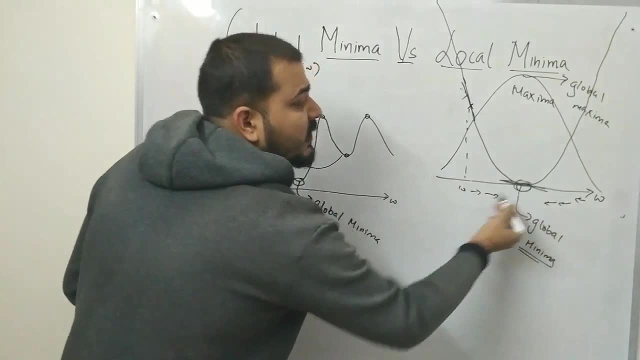 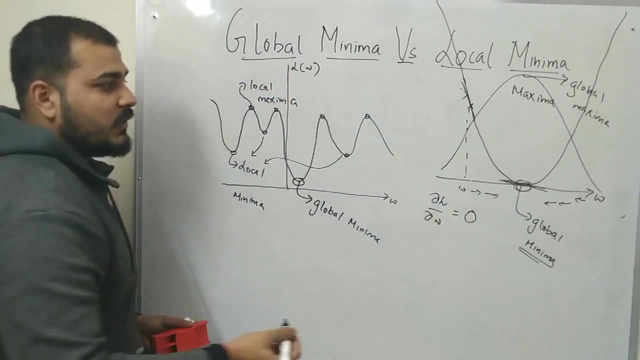 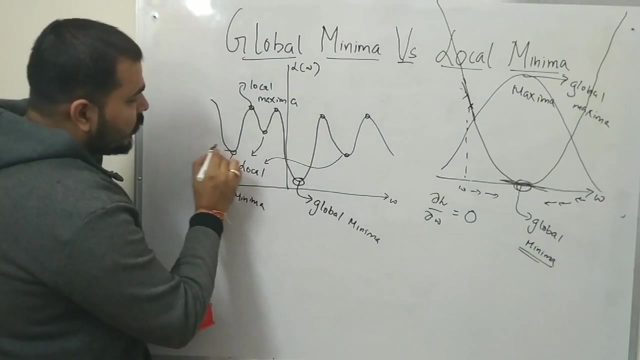 If I am trying to calculate the derivative at this specific point, Then the derivative of loss with respect to derivative of W will be 0. Because, you can understand, the slope for this kind of point Is actually 0. Right? Similarly, for this particular slope, it will be 0. 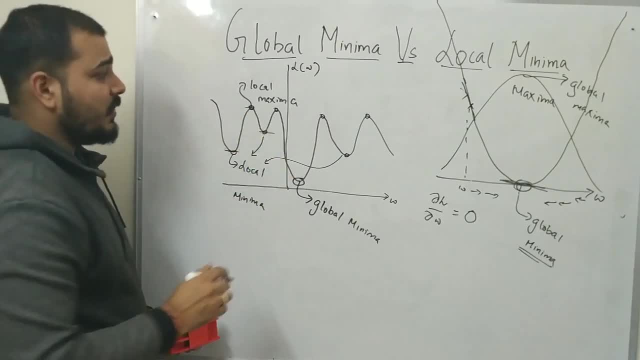 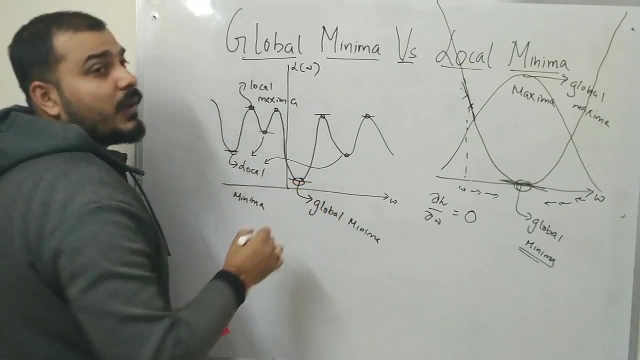 For this particular point also, it will be 0.. For this particular point, it will also be 0.. And for this particular point, it will be 0.. The reason it is 0: because the derivative for this particular point, Now the slope of this particular point, right. 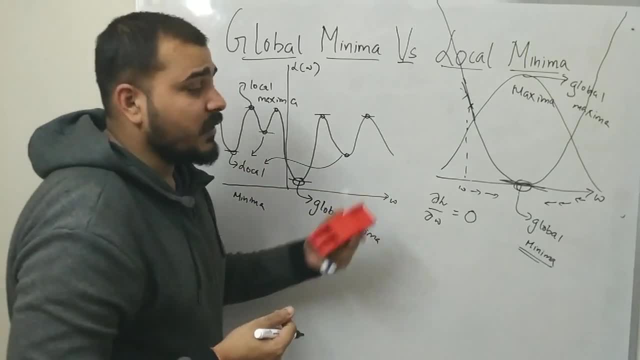 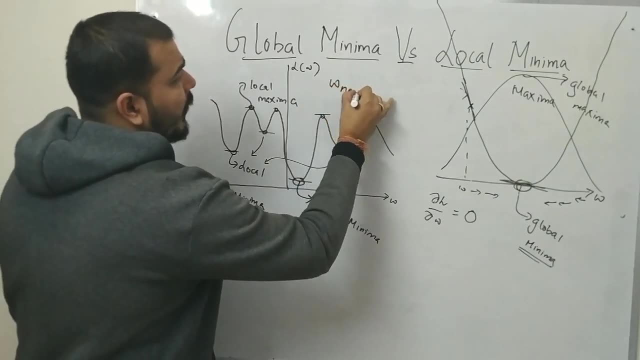 It is actually 0 if you go and compute it, And that is the property of this. Now, since it is 0. Since it is 0.. You remember our Y update Formula, right W, sorry, W update formula. How do we update the weight? 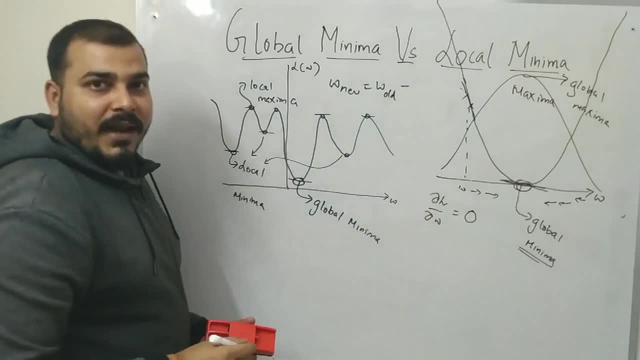 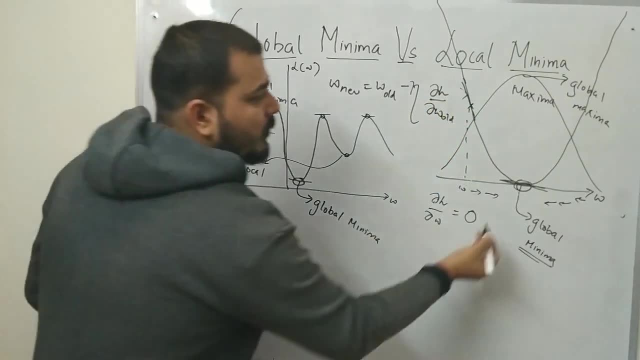 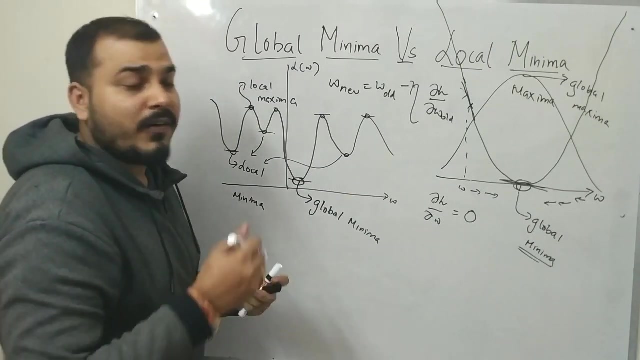 We basically write: W new is equal to W old minus learning rate Of derivative of loss with respect to W old. But just imagine if I come to this specific point, If I come to this specific point, And suppose your derivative of loss with respect to derivative of W old, 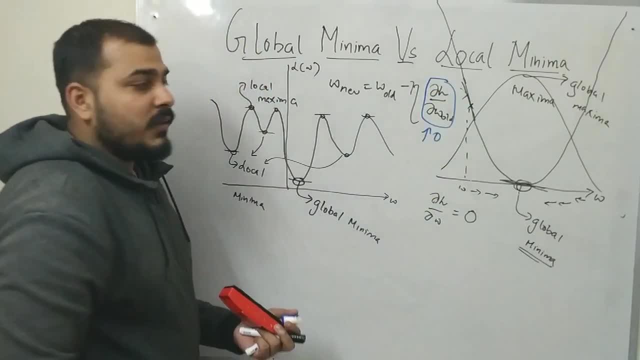 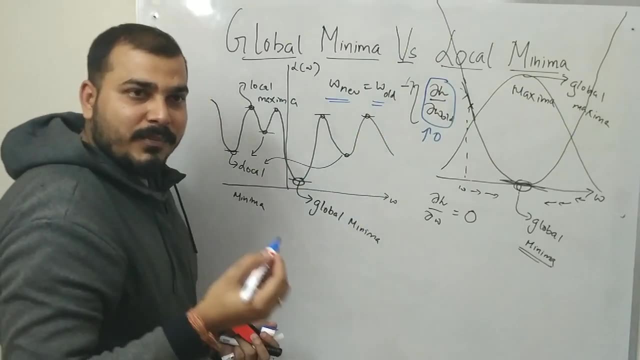 Becomes 0. if this becomes 0. Right, then that basically means this whole value will become 0. And at that particular point this W new will be equal to W old. That basically means that it has basically reached at this particular global minima point. 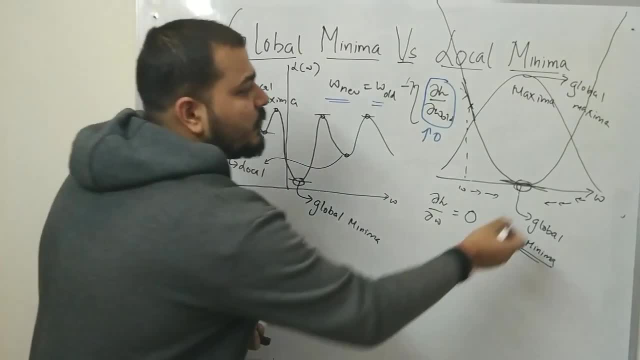 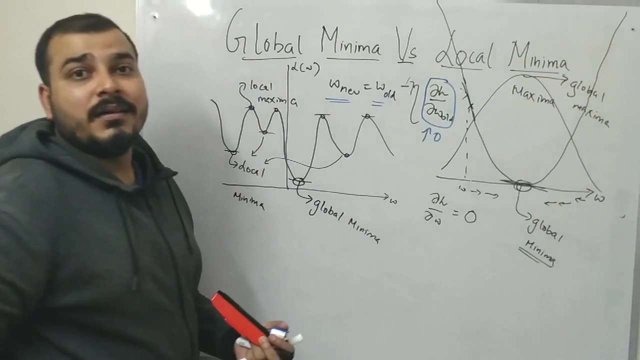 Since there is no update of weights, It will be treated as this. particular weights are the perfect weights For solving this particular problem. statement: Now, this is in the case of this kind of gradient descent curve. But what about this kind of gradient descent curve? 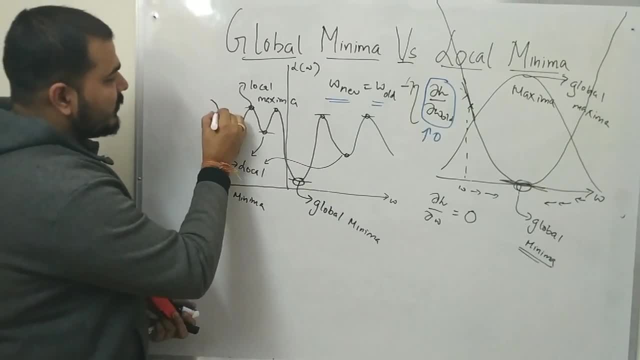 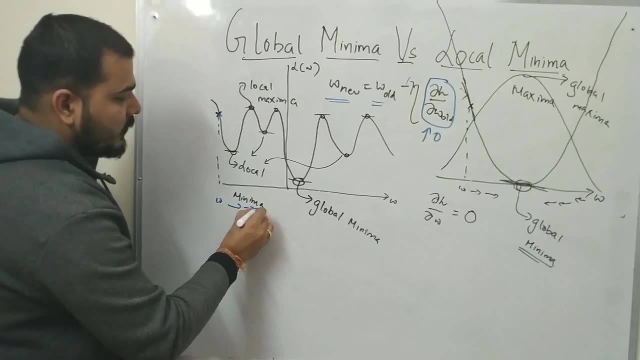 Okay, suppose my weights. initially it started from here, right, And we know that after I calculate a derivative of this, My weights will increase, right, It will come in this position slowly, slowly it will come down. Once it reaches this position, then again the slope will get calculated. 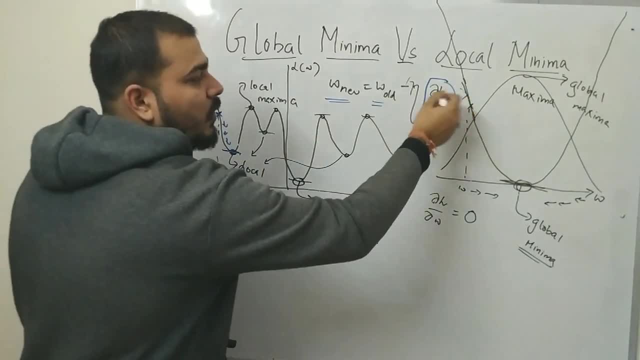 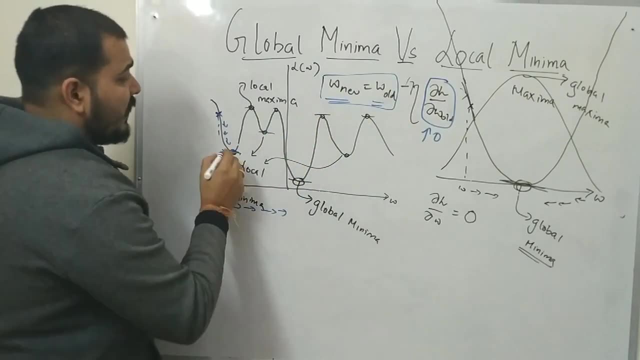 When the slope is getting calculated here, My slope will become 0 and this whole value will become 0. And W new and W old will become equal. Now the problem rises that I have still not reached my global minima. I am still there. 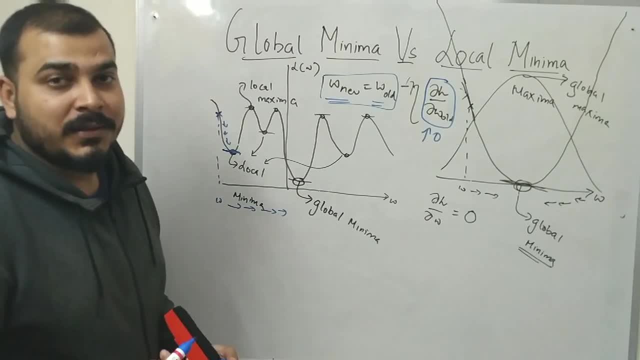 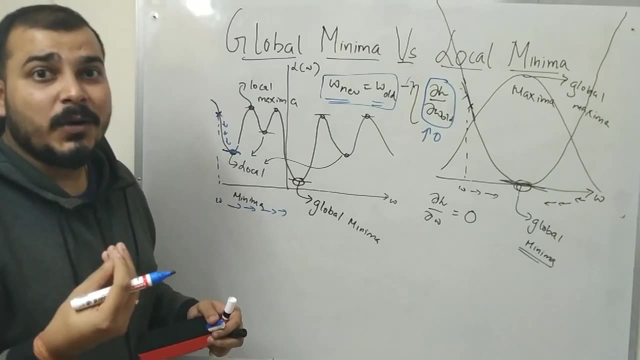 I am still there in my local minima, So what do I do for that? So this particular technique, I will be discussing in the next videos, Where I will be showing you some advanced techniques of optimizers, You know, and that will actually help you to prevent this local minima. 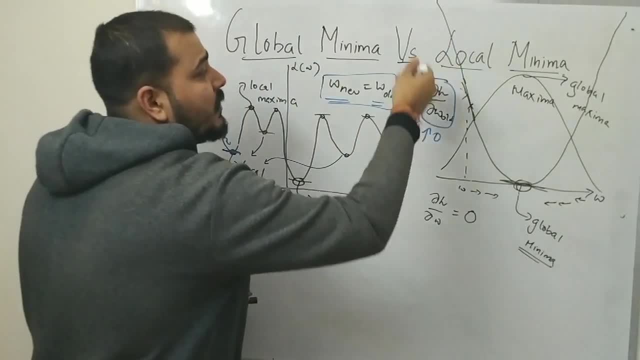 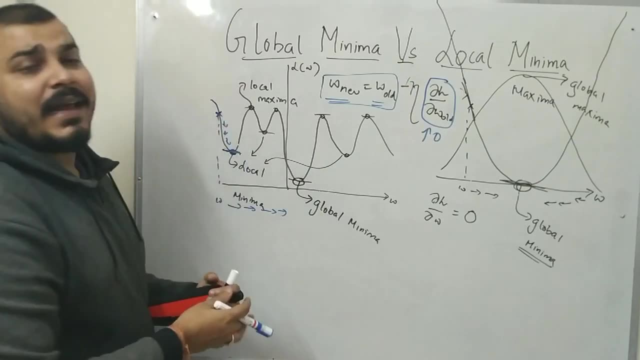 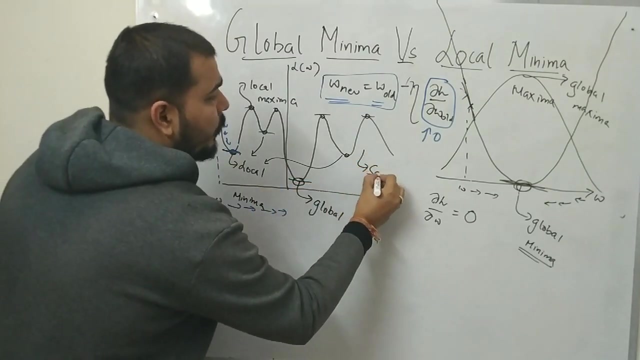 But you should understand the basic difference between what is a global minima And what is a local minima, and how it does vary. Okay, there is one more specific point that I want to discuss. in this global and local minima is that You will be having one situation which is called as saddled point. 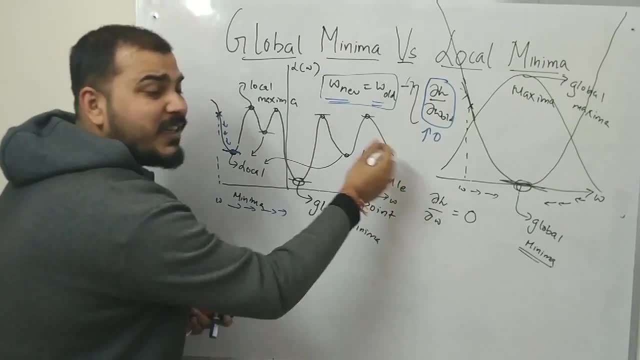 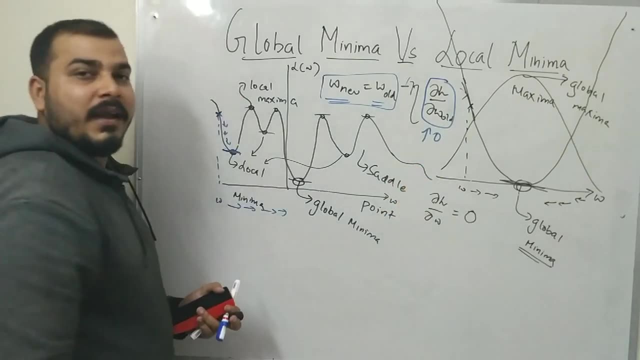 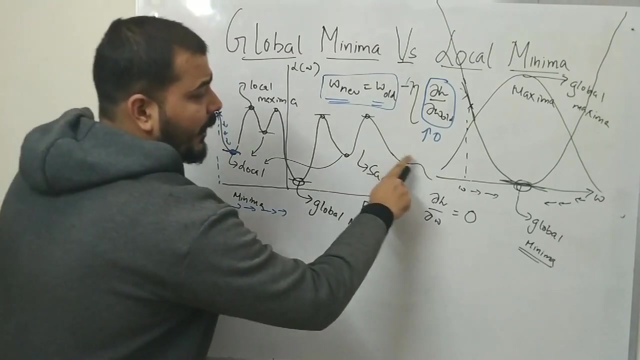 Which is called as saddled point. Now, what is this saddled point? you need to understand. Suppose, just consider that I have this kind of curve, right, I have this kind of extension of the curve. Now you observe that at this specific point, 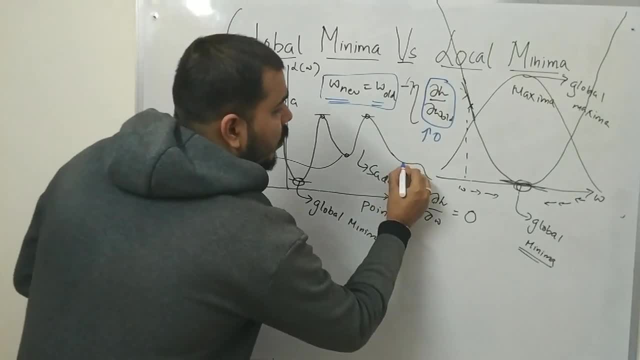 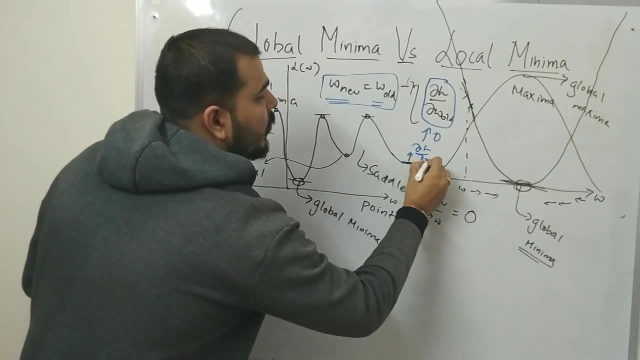 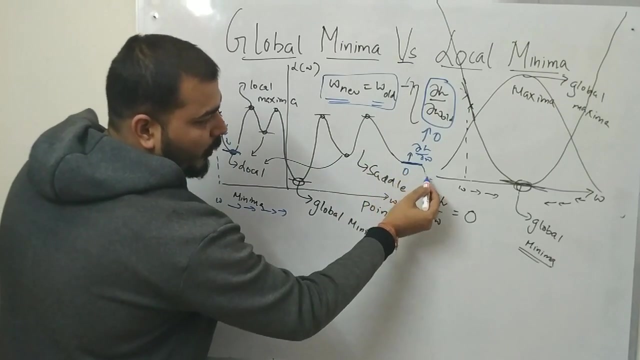 Whenever I calculate the slope, this also becomes 0.. Whenever I calculate the slope or the derivative with respect to weight, This will become 0, because you know that, right, This is just like one more local minima, But this particular point is reducing, it is coming down. 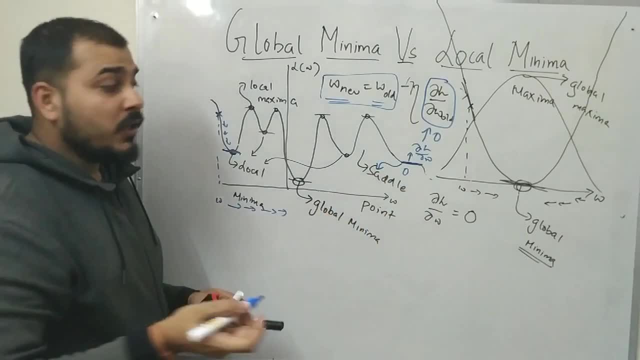 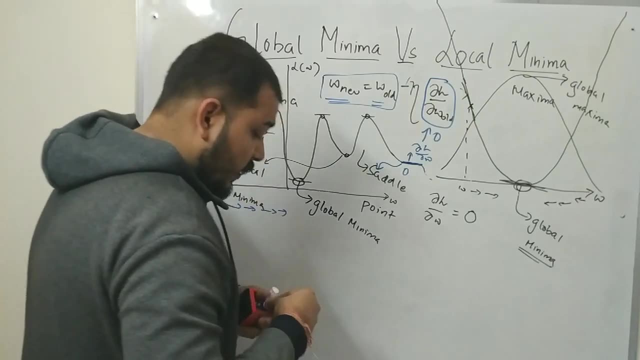 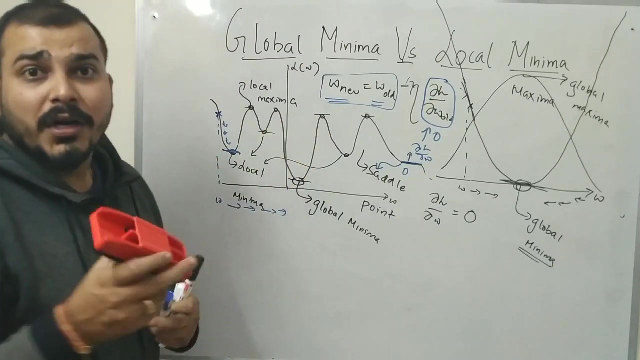 Right, and this kind of points are basically called as saddled point. So this kind of scenario will also come in some of the curves. Whenever we are discussing this Now, you may be thinking that why this kind of curves are actually present, right? So in order to do that, in order to understand that, we will be discussing about two functions. 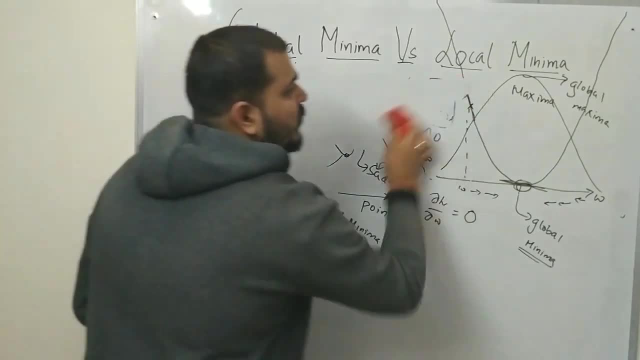 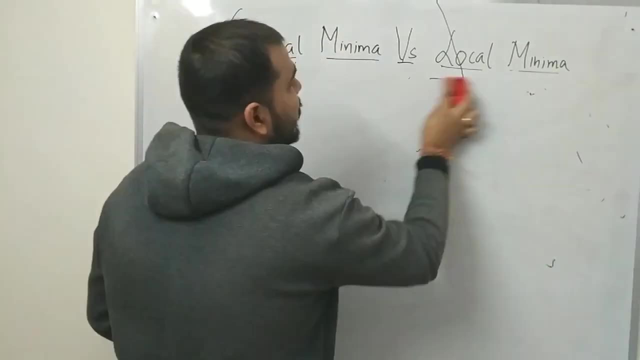 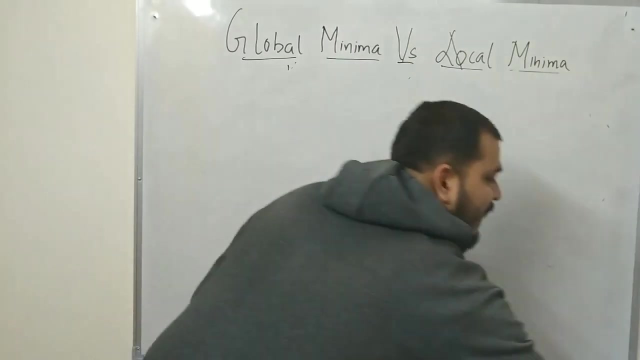 I will just rub this quickly. We will be discussing about two functions, and this two functions will actually make a lot of sense and you will basically be able to understand most of the things in that. OK, I am sorry for so much of scribbling and rubbing the board, but it is for your better. 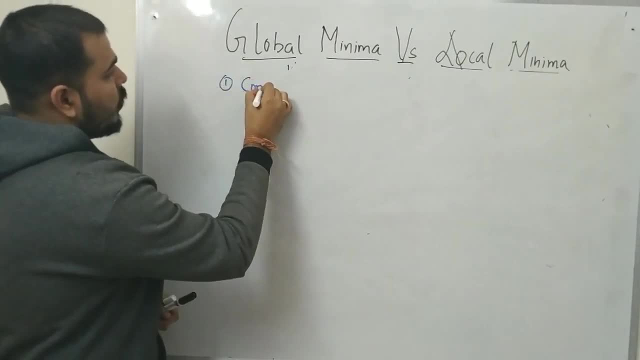 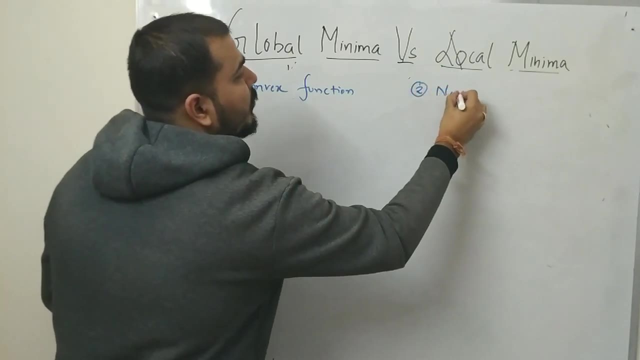 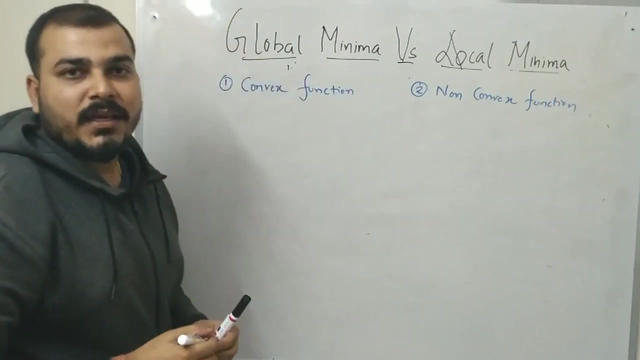 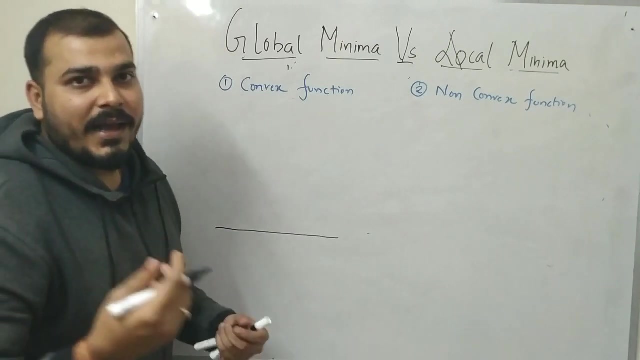 So I want to discuss about two functions. One is convex function And the second one is basically non-convex function. OK, So two topics: convex function and non-convex function. The example that I took with respect to our, you know, mean squared error gradient descent. 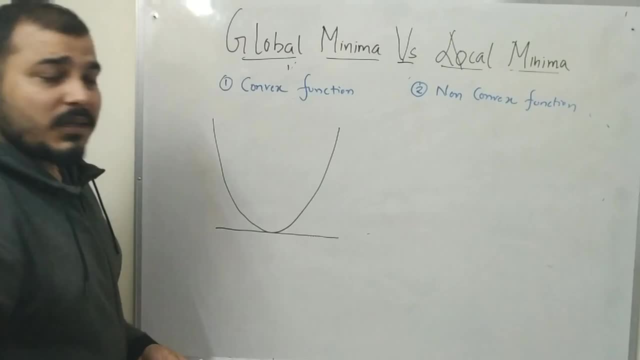 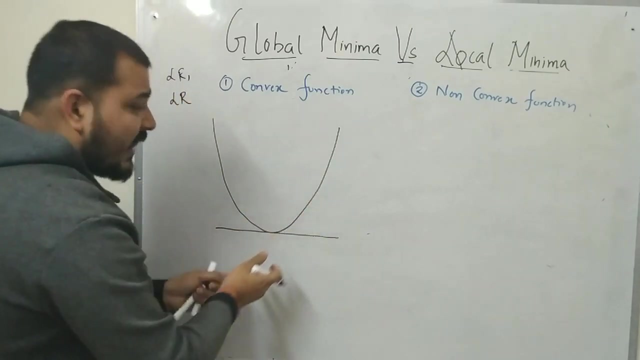 Where I had got this kind of curve. OK, This is an example of convex function. Now, this kind of gradient descent occurs in most of the machine learning problems. There are some statements like linear regression, logistic regression, Right. So there you will be, seeing that this kind of curve usually happens. 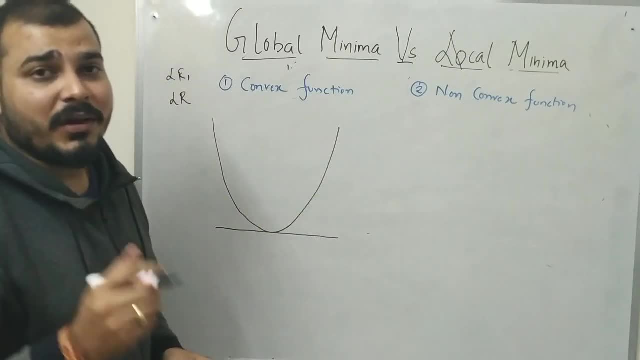 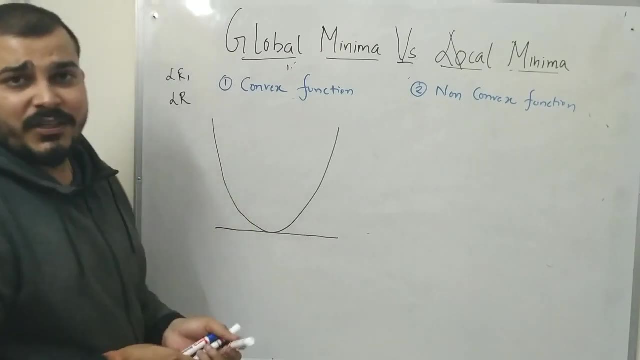 But this kind of curve will not be exactly present in deep learning. In deep learning you will be having some non-convex function kind of curves. Now, first of all, let us understand what is this convex function? So understand, guys, in this convex function. I can divide this whole area into two parts. 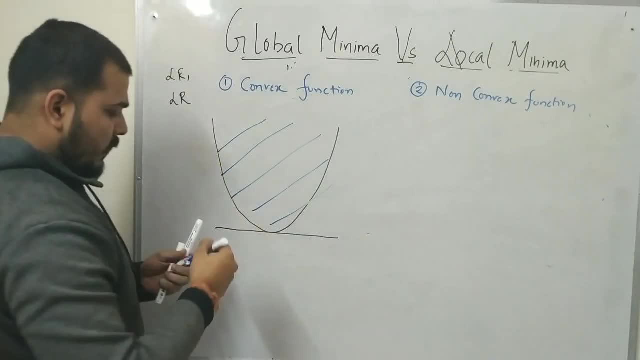 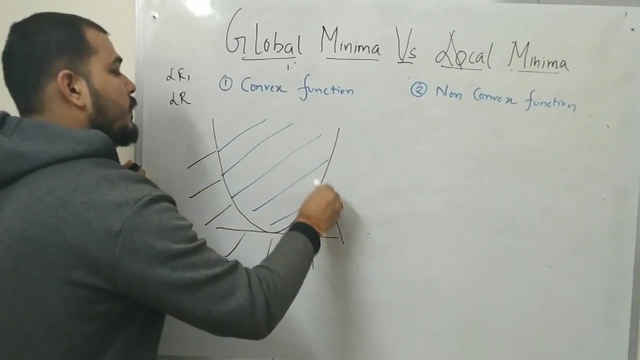 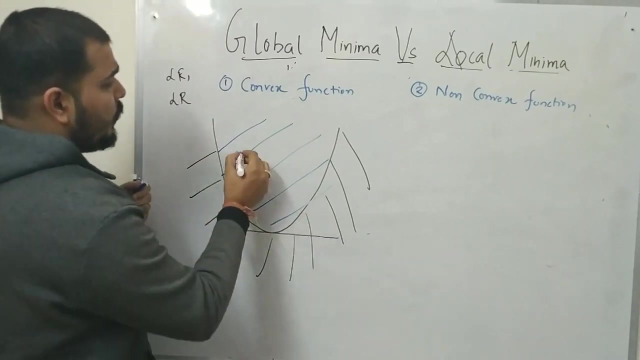 This will be one area, OK, And the other area will be somewhere like over here. So this will be my second area, Right? So how do I decide how many areas are there? That basically means that suppose I consider two points, Two points anywhere in this side this curve. 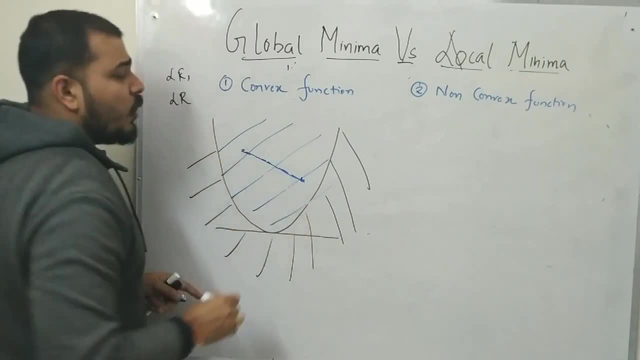 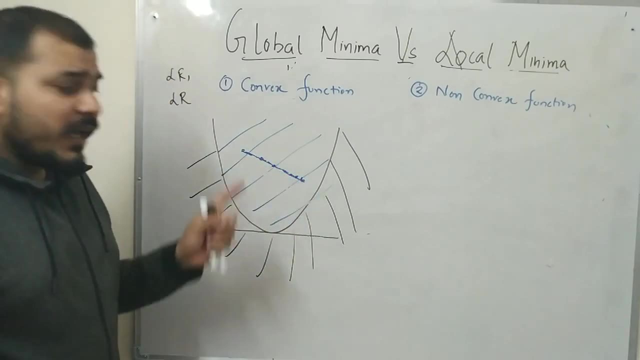 And if I try to connect it, If I connect it, I will go and see that whether all these points from which I have connected is present in the same curve or not. So if it is present in the same curve, that basically means that it belongs to convex function. 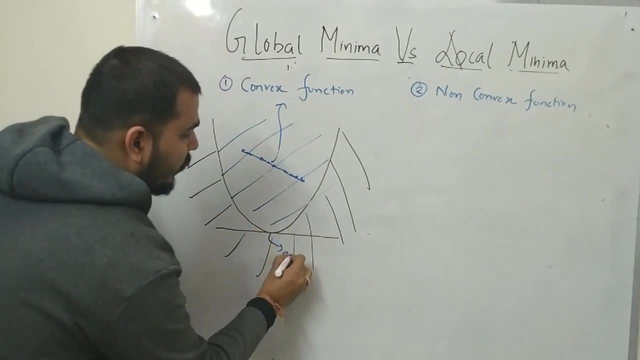 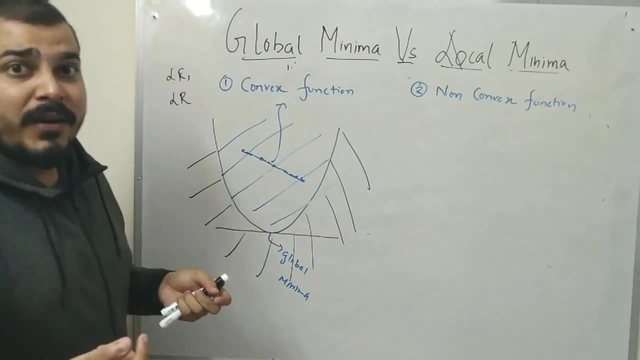 Always remember in your convex function, you will be having only one global minima. You will be having one global minima, OK, And about the maxima: it may be present. at least one maxima may be present. sorry, not at least one maxima may be present or it may not be present. 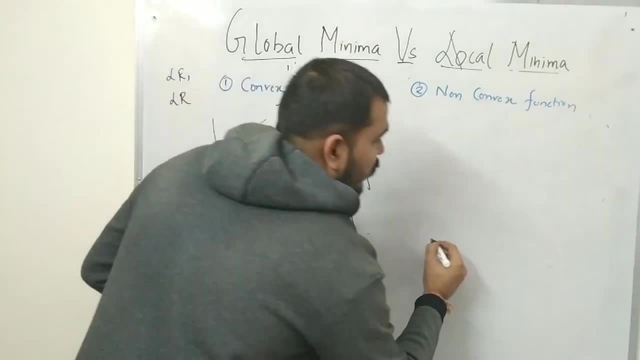 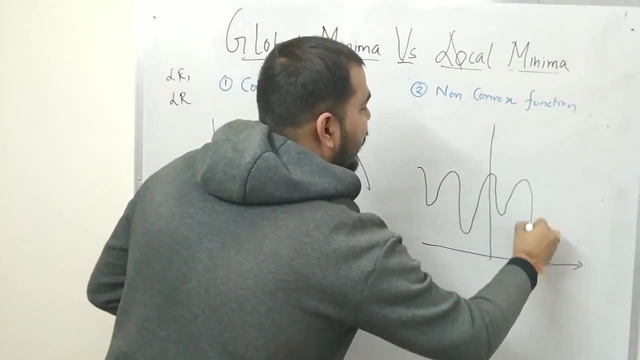 The next thing is that let me just give you an example of non-convex function. So non-convex function we have already discussed Again. I will just draw the same hyper parallel. I mean this type of local minima and global minima. 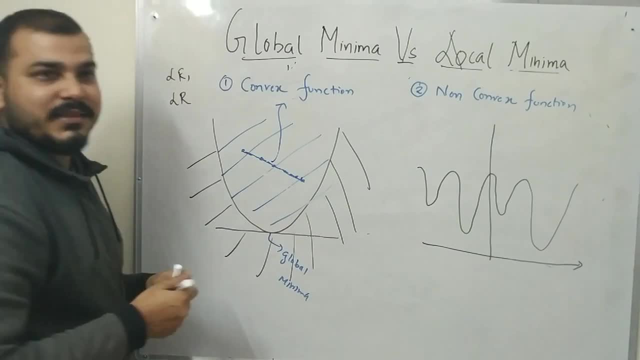 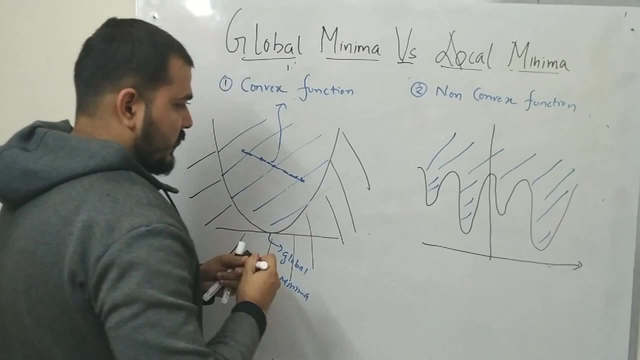 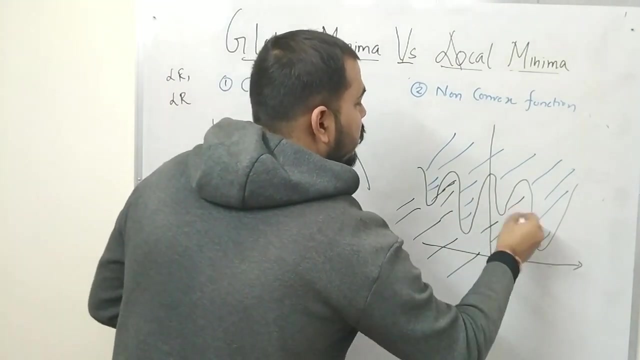 Over here. just understand again. I will try to divide this into various regions. Suppose this is one of my region And this second part will be my region over here. Right? So two regions have been changed. Now what we will do is that we will consider two points. 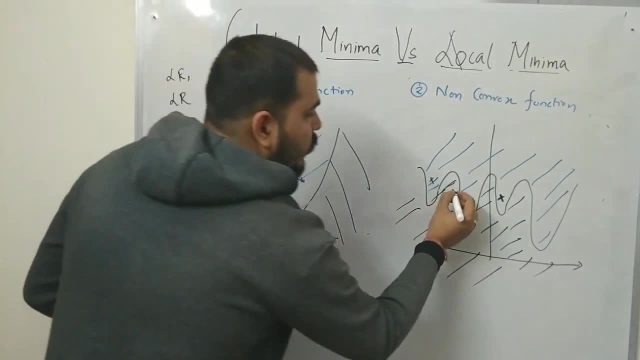 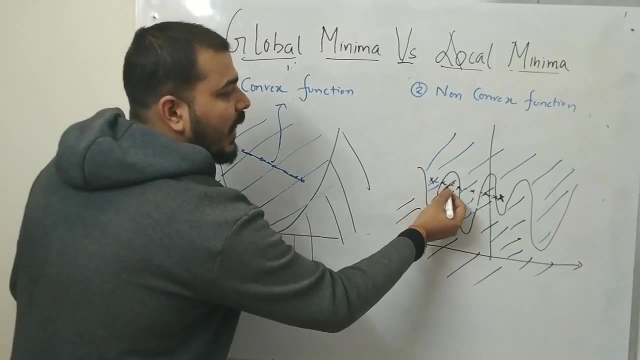 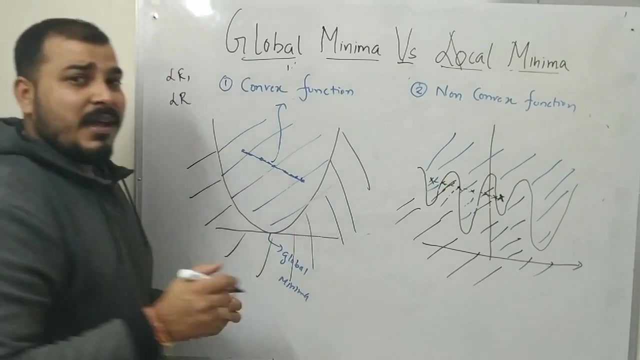 This will be my one point and this will be my another point. Now, if I try to join all these points, then we can observe that these all points are present in two, two regions. It is not present in single regions like this Right. So this is the basic difference. and non-convex function usually occurs in most of the deep learning techniques. 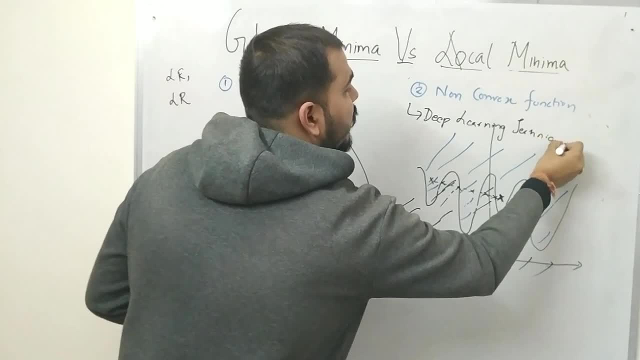 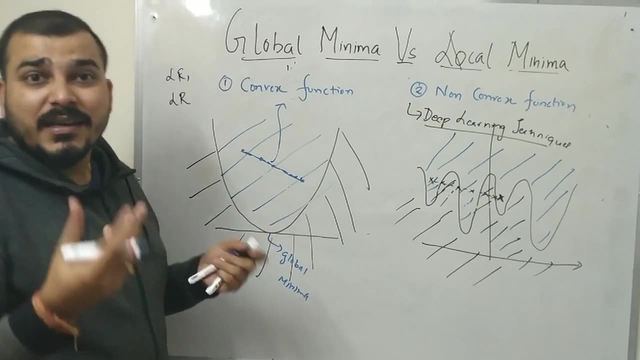 Most of the deep learning techniques. You know this kind of situation. it will be present in deep learning techniques. And why it will be present? because, understand, there are so many weights parameters, There are so many neurons that we are using and each and every neuron needs to get converged.